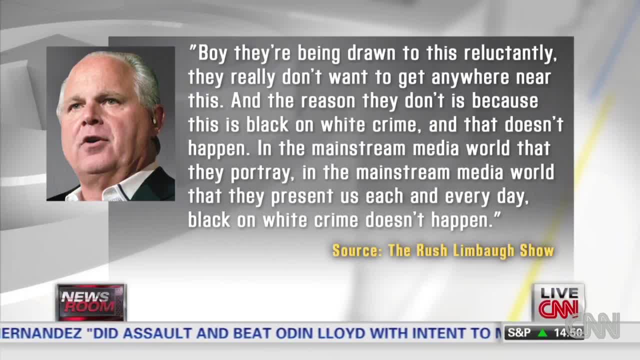 And the reason they don't is because this is black-on-white crime And that doesn't happen In the mainstream media world that they portray. in the mainstream media world that they present us each and every day, black-on-white crime doesn't happen. 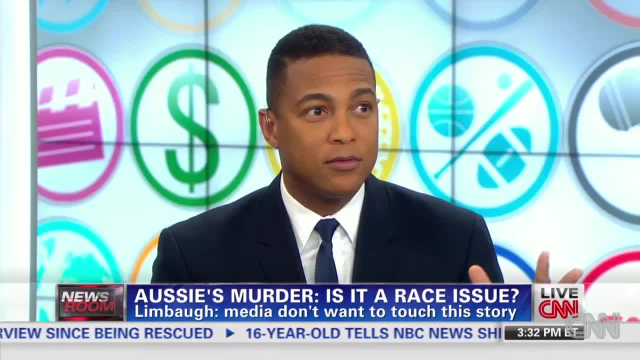 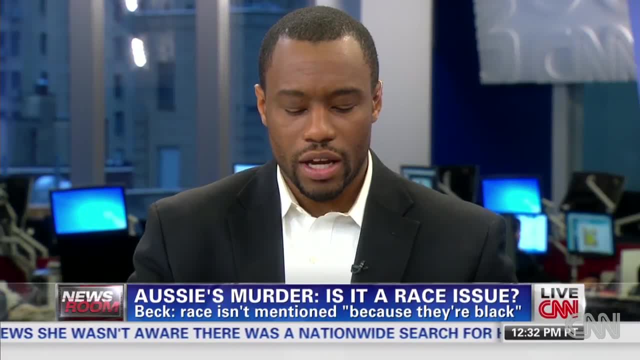 They have a point that Trayvon Martin race became an issue in this, but this didn't. Do they have a point? No, they don't have a point. First of all, the media. The media coverage on this has been probably more intense than it was on Trayvon right after it happened. 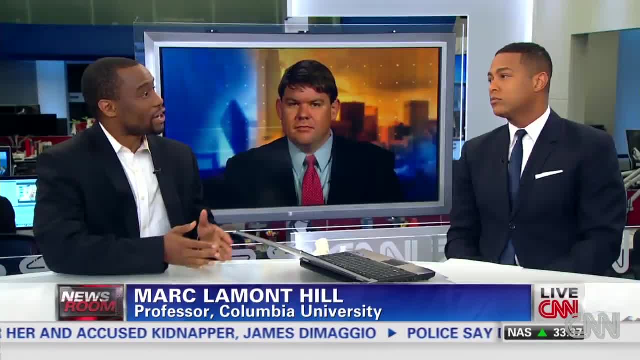 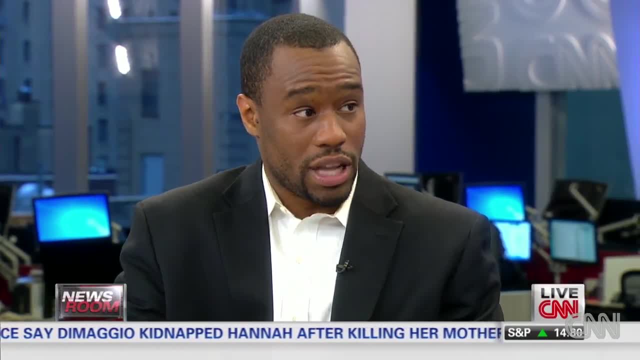 It took months for the Trayvon Martin controversy to come to the national media and it only came to the national media Because he wasn't arrested, Because there was no arrest, because there was so much dysfunction in the process. Here the alleged killers have been arrested, they've been charged. 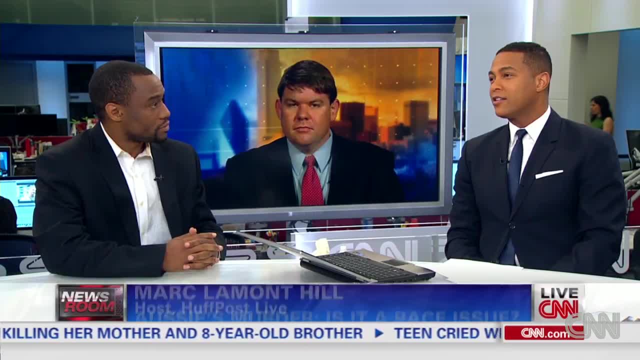 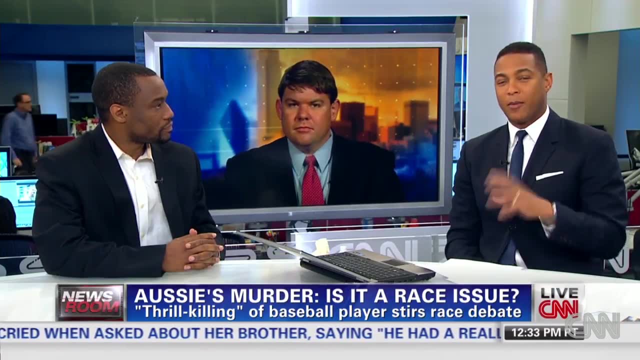 If this had happened with Trayvon, we wouldn't even know who Trayvon was, Is that? But many will say that is making an excuse, because race is a third rail in this country And anyone who is, if you're talking about it. if it had been three white guys. 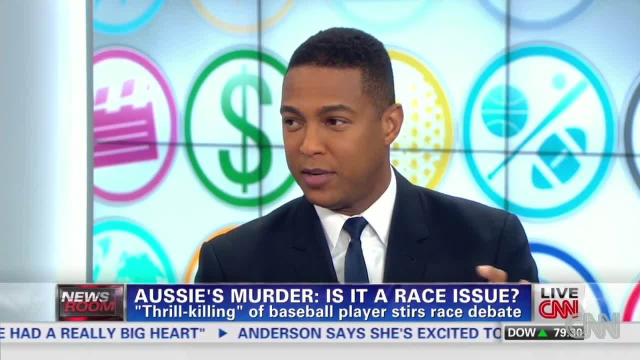 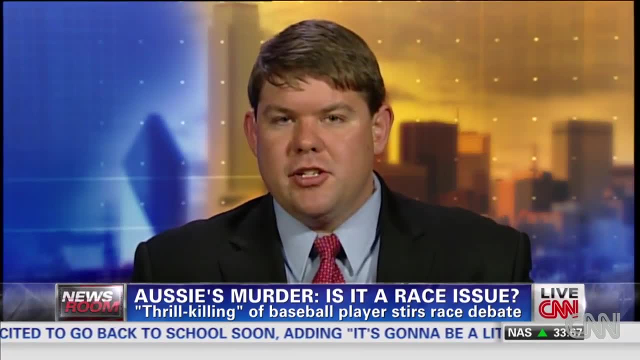 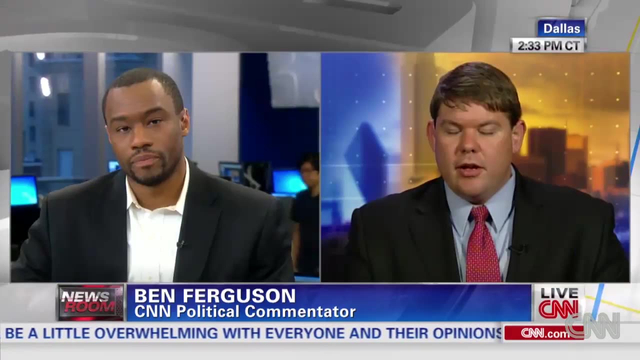 and he had done that to a black guy immediately, the media would have jumped to race Ben Ferguson, go ahead. Yeah well, not only that, but you would have had Jesse Jackson, Al Sharpton and many other leaders out there that would be doing exactly what they did with Trayvon Martin. 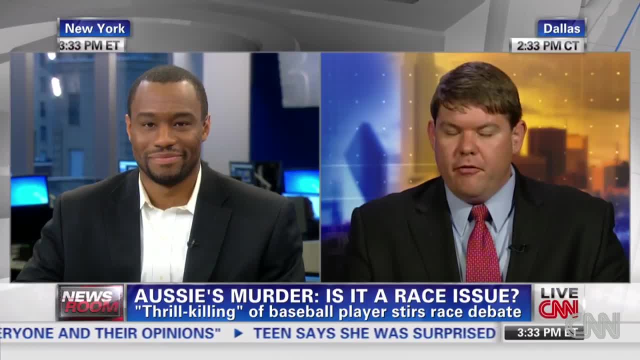 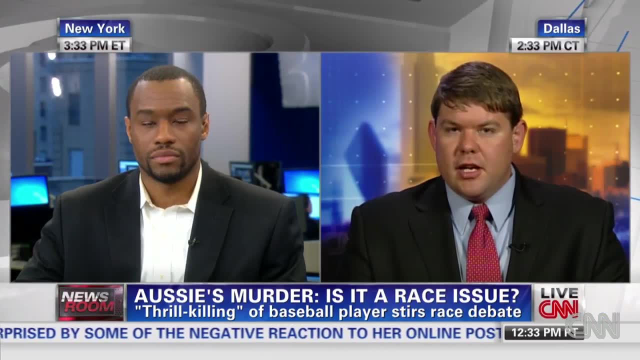 And in this case it's a white kid that's profiled. We now know from some of the tweets from one of the guys that had the gun that he said white people disgust me, And another time he said I hate all white people. 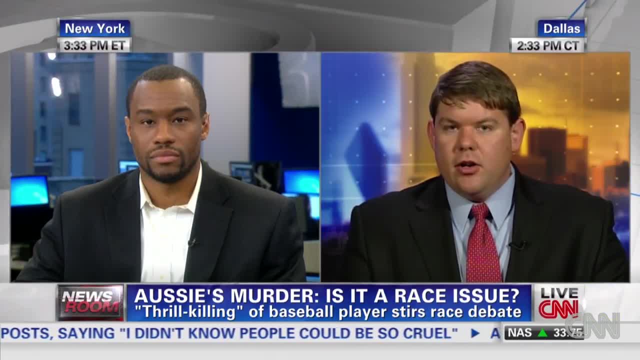 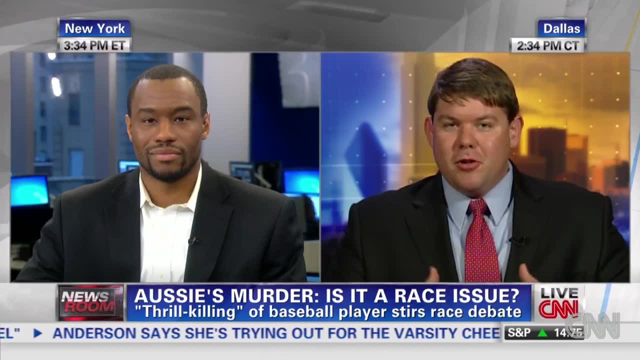 And there was multiple tweets based on race in there dropping the N-word and then saying I've got the whiteys and that kind of thing. This is a crime that it's pretty obvious had some racial implications to it truly. 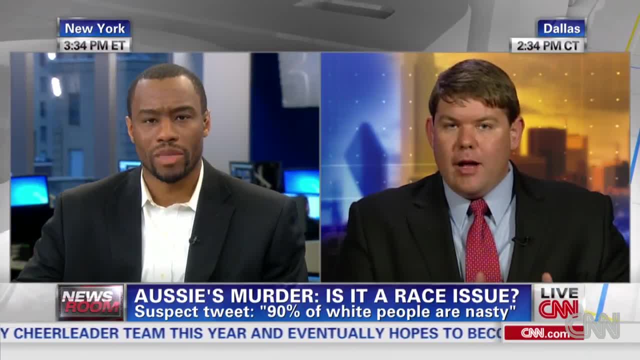 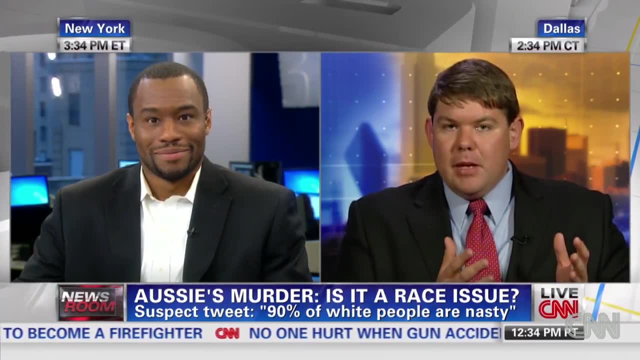 By those that did the crime. they go out and find a random white person who's running and kill him. How does race not be a part of this, And even the issue of can it be a hate crime? I have yet to meet anybody who says: 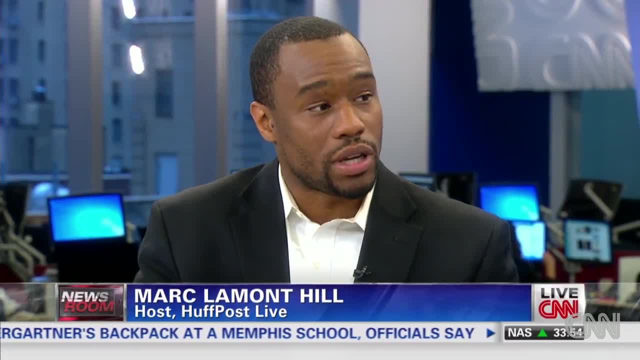 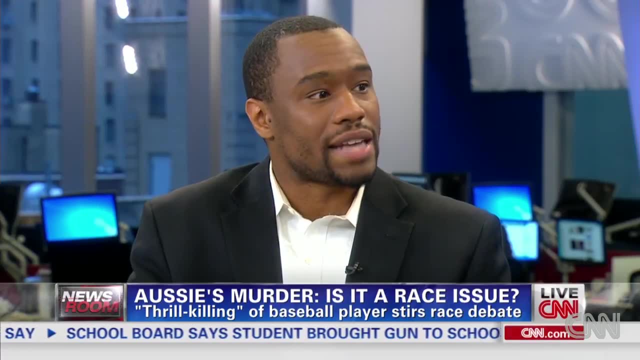 It says that killing a white person isn't a hate crime. I have not met anyone who has said that this wasn't driven by race. They said: we're going to kill a white person That is by race. If that is in fact the case, it's a race crime. it's a hate crime. 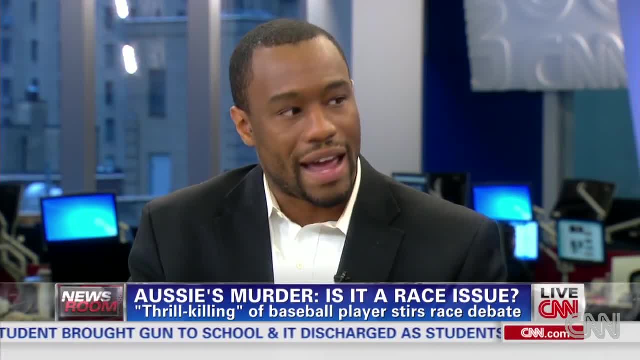 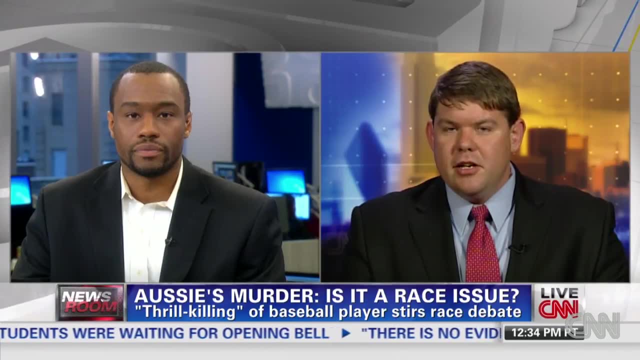 That's not the issue. The issue here is if there's a double standard or not. And there is not a double standard, And there is, I think there is White people, And here's the difference. How, Ben? Here's the difference. 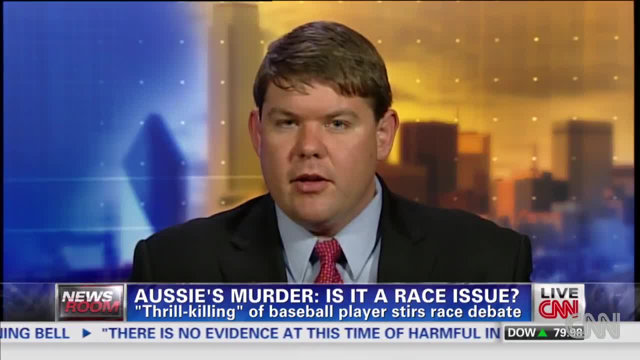 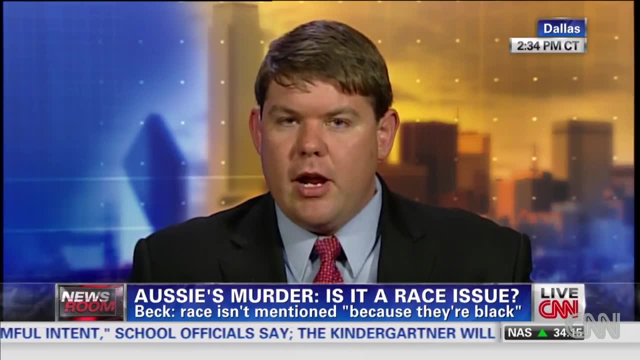 When you have something like Trayvon Martin that comes out, and you have marches, and you have pastors, and you have people that are going out there and all they're doing is beating on race, race, race, And then the same exact thing happens. 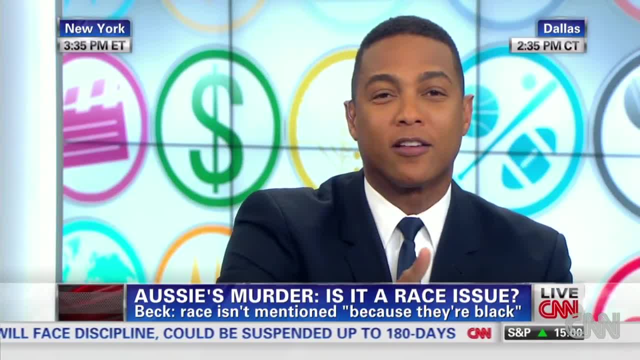 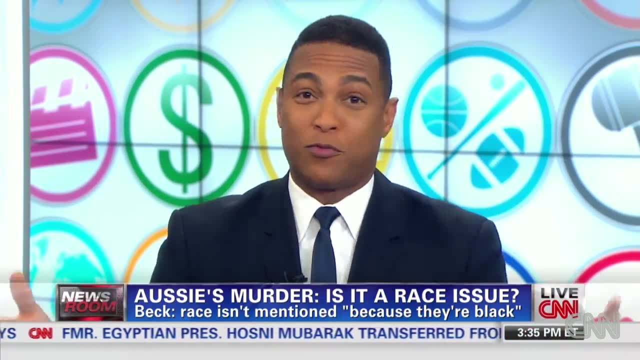 And Ben, let's do point by point here. Let's do point by point. So you said you have pastors coming out. No one's stopping white pastors from coming out and saying anything about it. if it is So, white pastors can have the opportunity to come out if they want to. Ben. 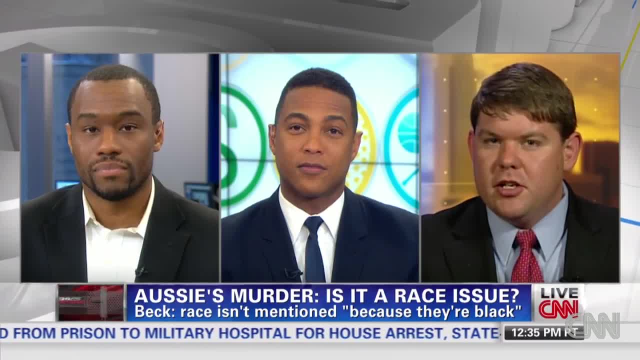 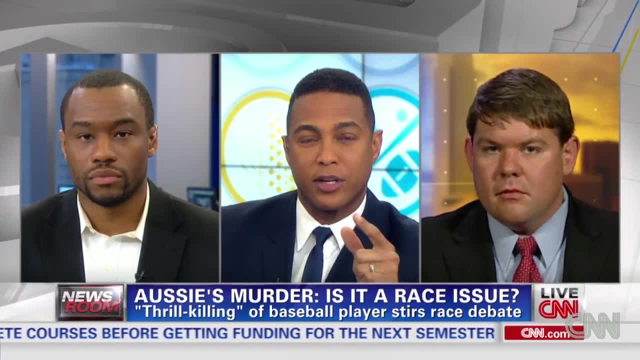 And who would cover that? And, more importantly, they would say they're out of touch. and well, they're racist because they're coming out having some white march. We have white pastors coming out. It's a double standard. James Edwards, the youngest of the three, tweeted this that he and his friends were ready to take some lives. 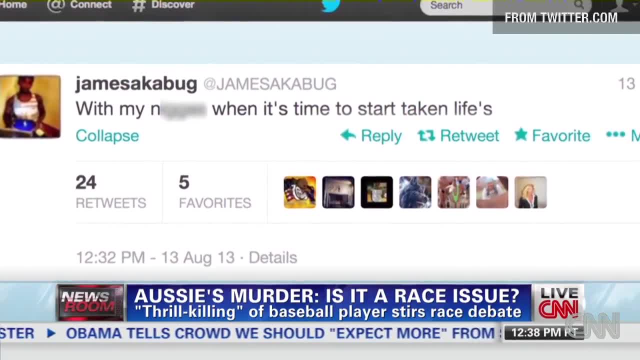 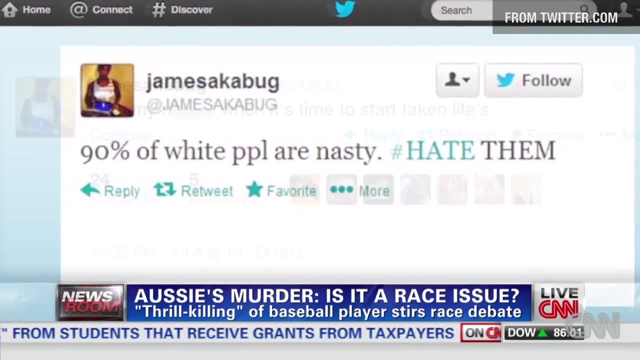 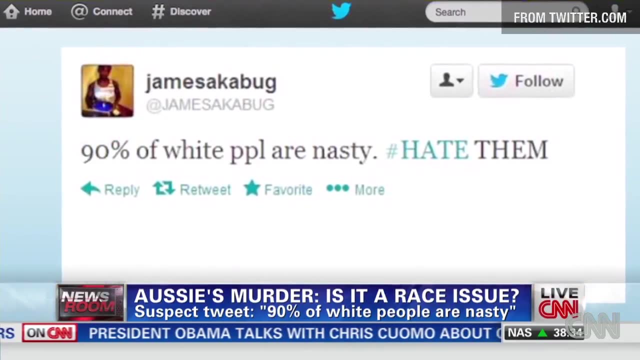 Back in April he posted: 90% of white people are nasty. He posted rap videos and talked about being a gangster. What does this say about the culture and the kind of people or person he might be In conjunction with the acts that he allegedly committed? they say a lot. 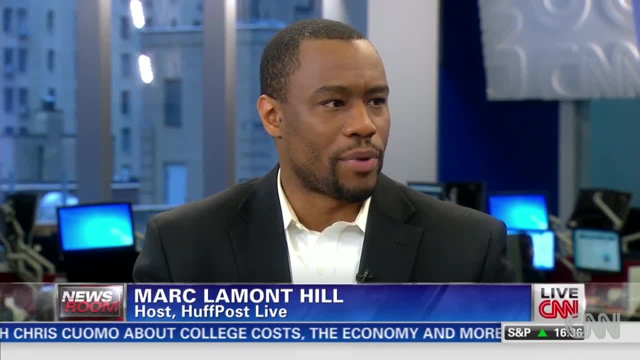 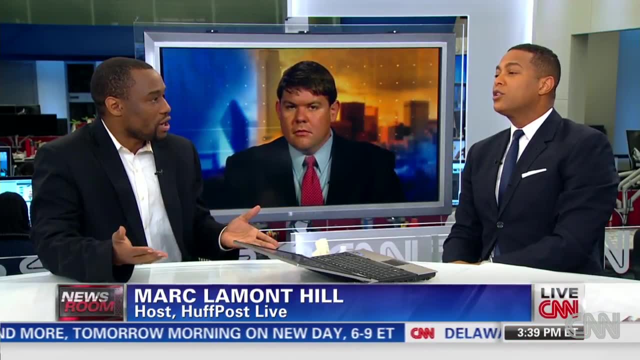 But there's no way ahead of time that we could look at someone who celebrates rap music and do some criminalization. If we did that, we'd be intervening on half of America and many young white people in the suburbs. But you don't think that the media would be jumping on this if, let's say, the situation was reversed. 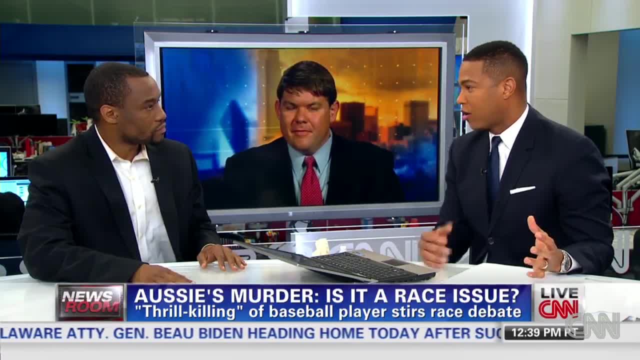 and they'd say: oh well, 90% of black people are bad and we're going to go out and kill people. I think people would look at that as a sign of something problematic and they would use that as evidence for a hate crime. 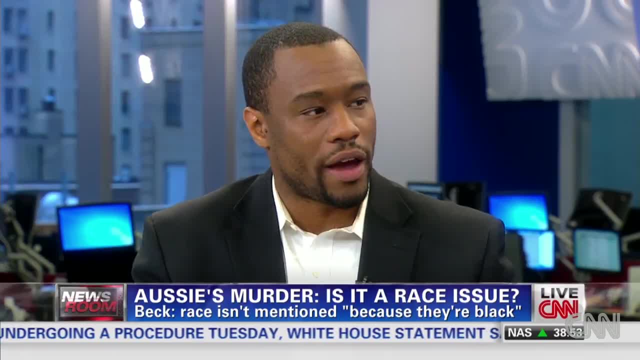 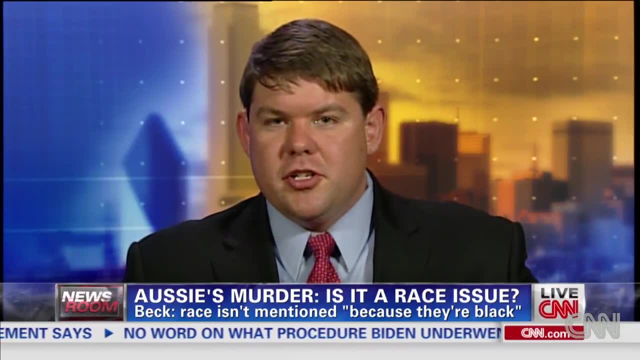 I think the same thing should happen here. All I'm saying is: a week after the murder, it's too early to say that we haven't done it. That's all I'm saying. Then I've got to go quickly. Here's the core issue. 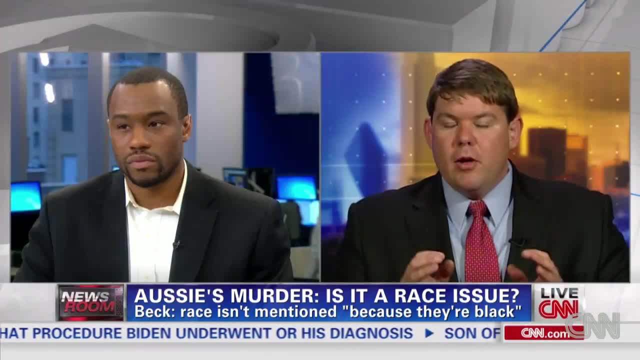 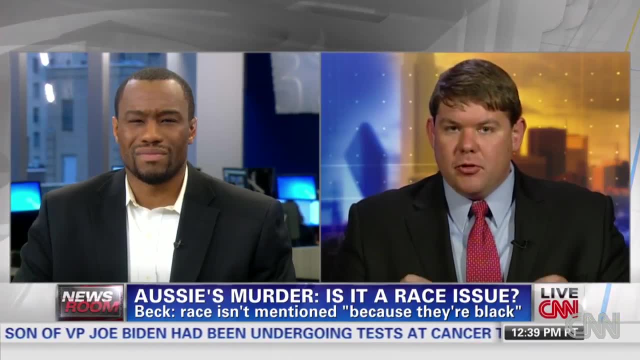 If this would have been switched and those tweets would have gone out, we would have had the first charge be a hate crime. and there still has not been a hate crime charge to any of these three people. That is the double standard at its core.